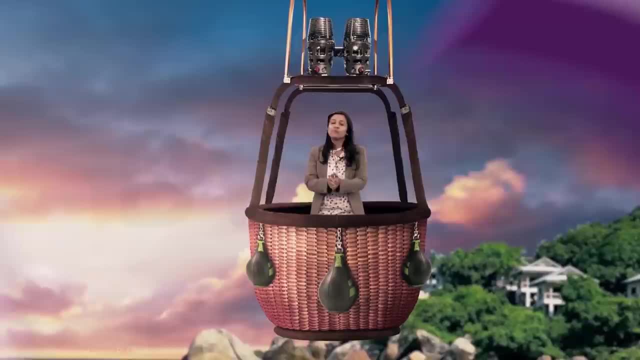 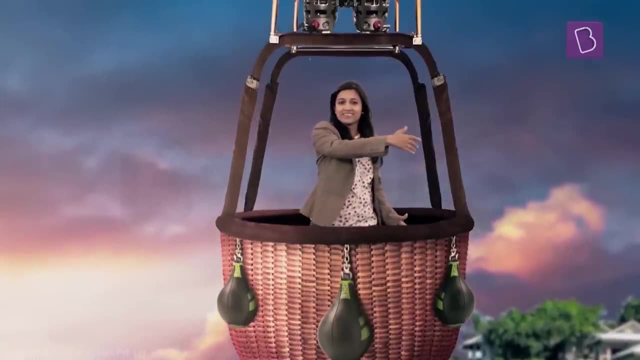 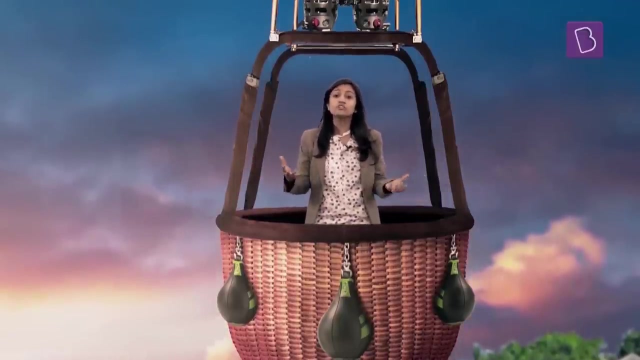 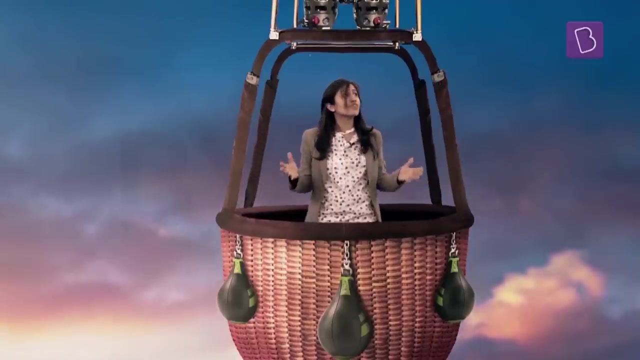 So we have this special substance that floats around on earth, Something that you cannot see, but you can feel it, You can swish your hand through it and, most importantly, it allows all of us on earth to breathe air. We give a fancier name to this blanket of air that surrounds the earth: We call it the atmosphere. 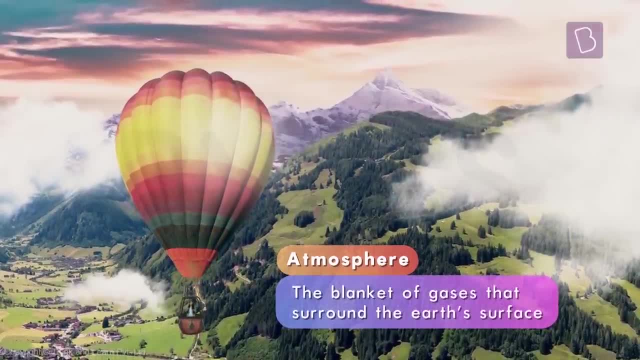 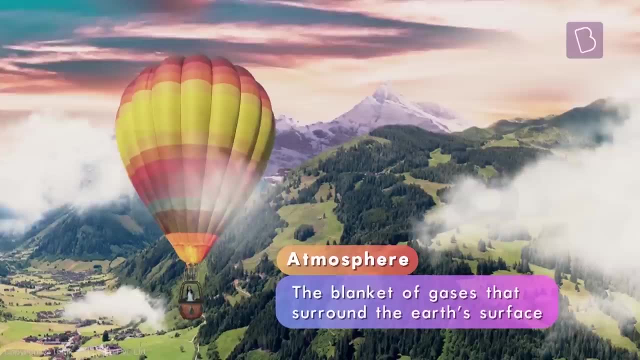 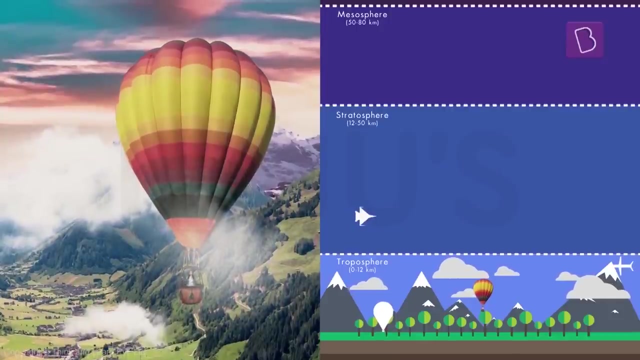 And much like a blanket that you snuggle under to feel nice and warm. the earth's blanket also has a role to play in keeping the earth's temperature in place. This blanket- the earth's atmosphere- has many, many gases in it that are necessary for us to be alive. 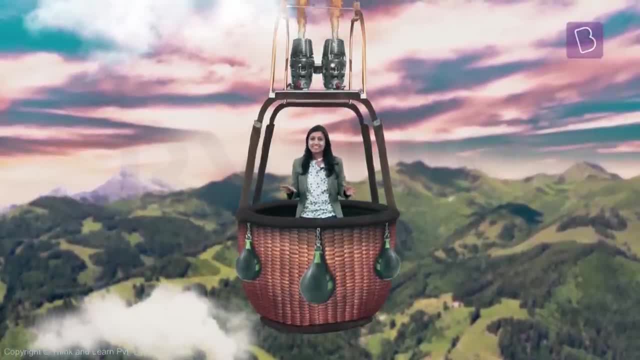 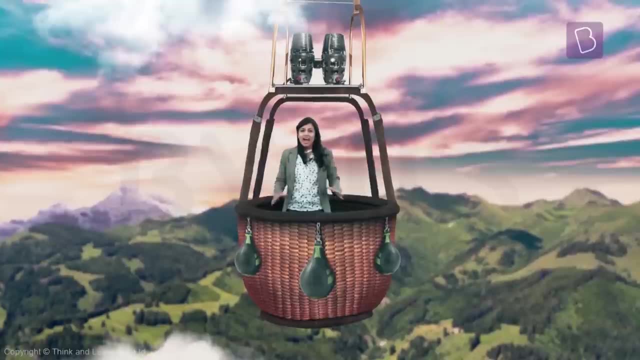 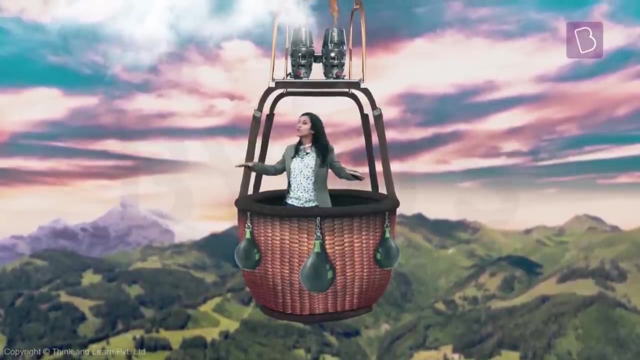 Also, something really interesting is that the part near the surface of the earth That's about to explode, The part near the surface of the earth where we are, has more air than the parts above where we are going to go. This part of the earth where we are floating about now has the maximum amount of air. It's called the troposphere. 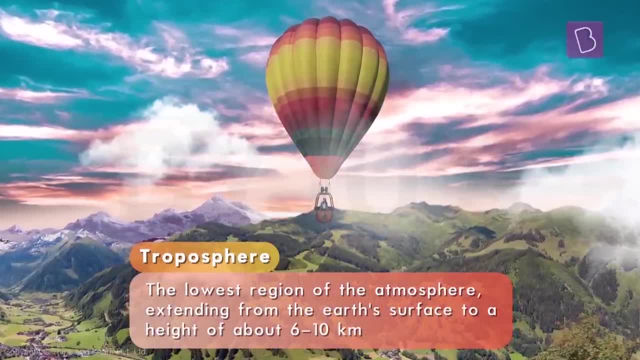 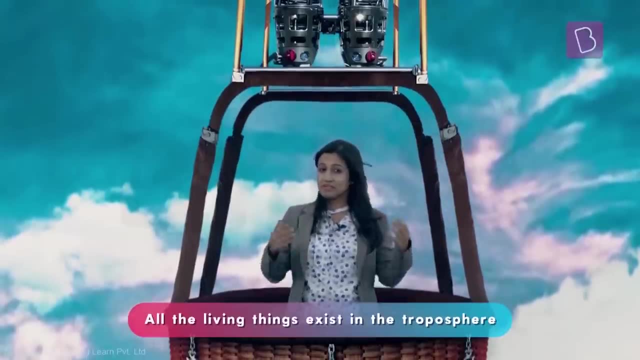 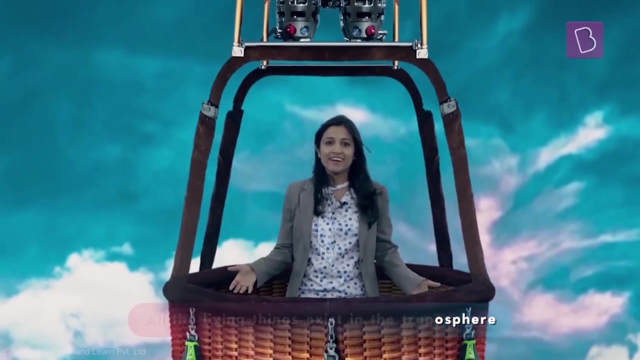 It starts from the surface of the earth till about 10 kilometers above the earth. All the living things you see, like animals, birds and insects, and even some non-living things Like clouds, exist in this layer. The troposphere contains 75% of all the air. 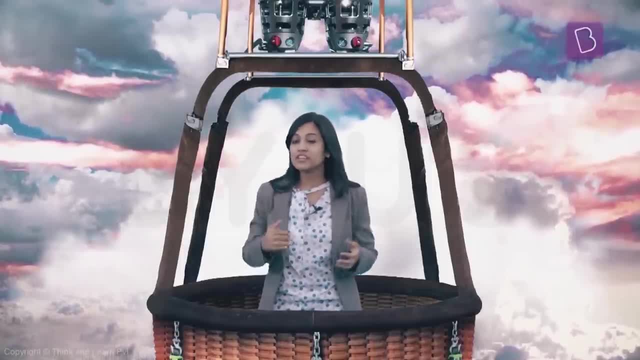 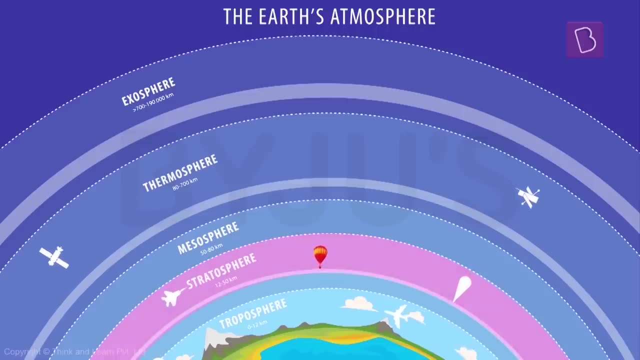 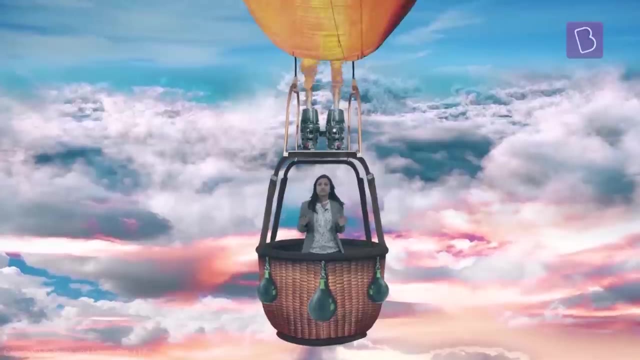 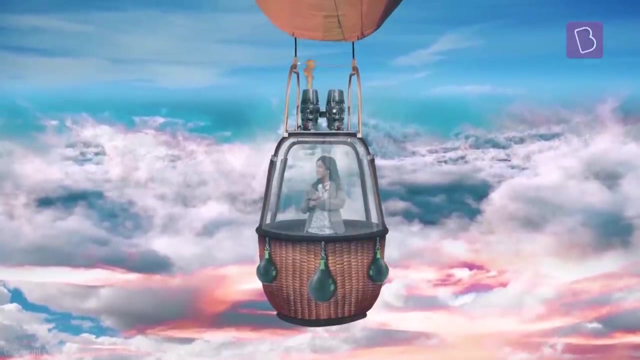 As we start going higher up, the air starts to get thinner On to the next layer of the atmosphere. Welcome to the stratosphere. It is very cold over here and there is very less oxygen. I have enough oxygen right now. Let me just turn up the temperature as well. 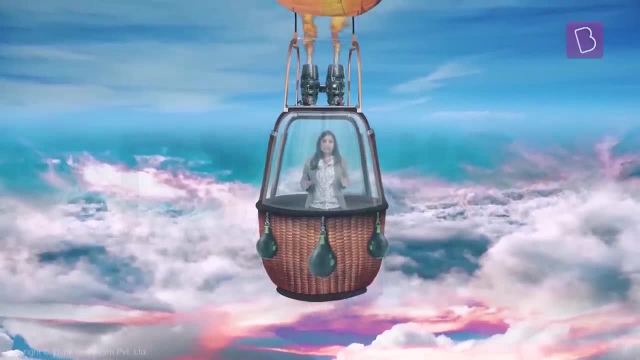 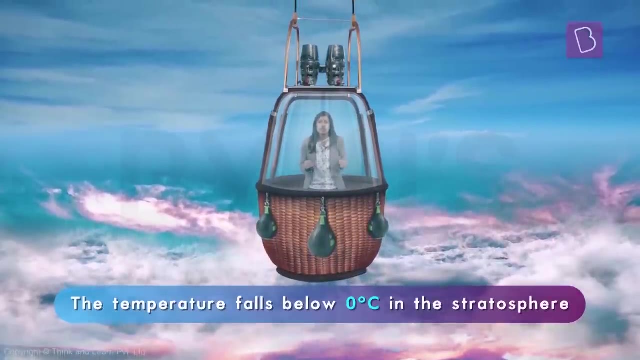 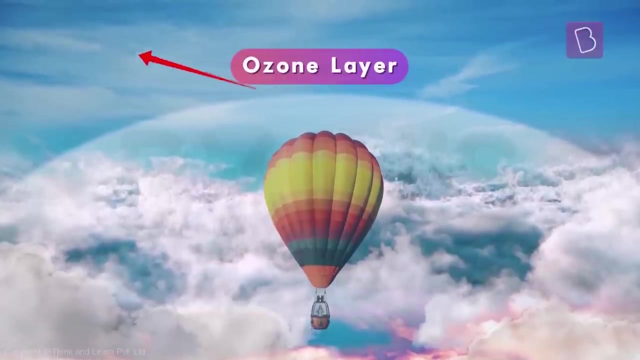 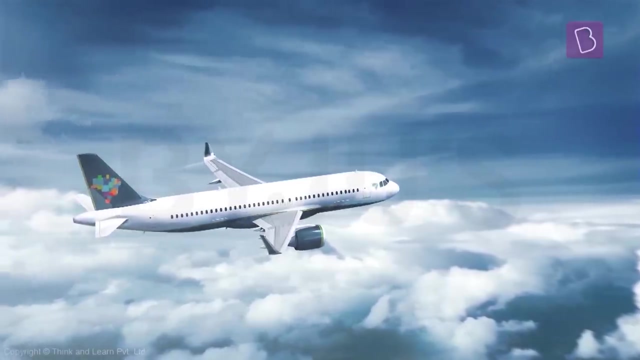 Perfect, So it gets very cold in this region, with temperatures going below zero degrees. This region holds something called the layer of ozone. Now, ozone is something that protects all beings on earth from harmful UV rays of the sun. Think of an aeroplane as a cylinder filled with air and sealed tightly so that air does not leak.